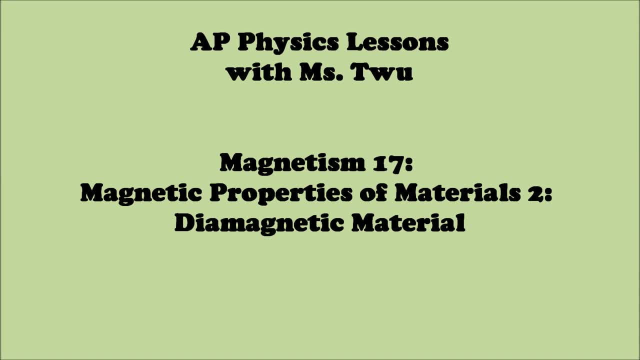 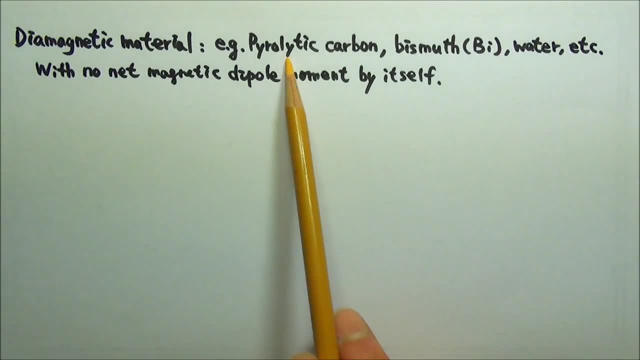 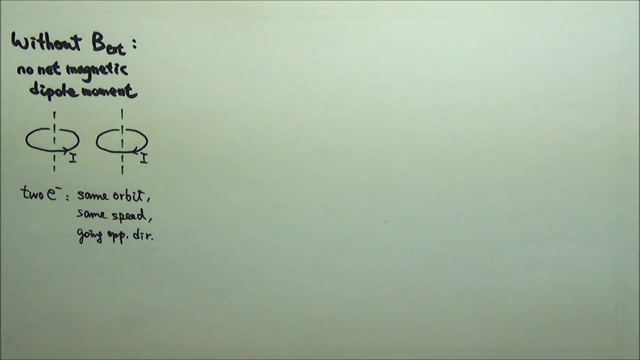 In diamagnetic materials such as pyrolytic carbon, bismuth and water. the magnetic dipole moments by all electrons in a molecule cancel each other, So it has no net magnetic dipole moment by itself. We will use classical model to illustrate things again. Let's consider two electrons. 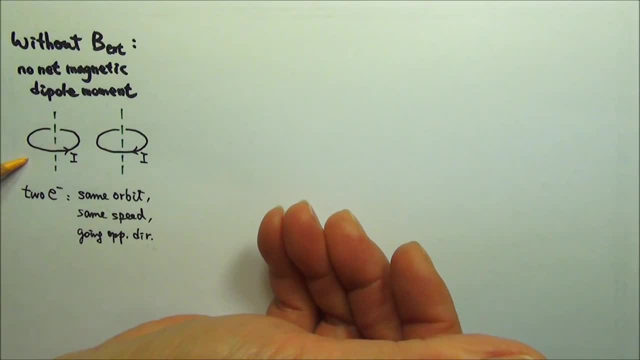 For this loop. when I use my thumb to follow the current in the front, my curved four fingers point upward inside the loop. So this electron's magnetic moment goes up, that electron's magnetic moment goes down and their net magnetic moment is zero. 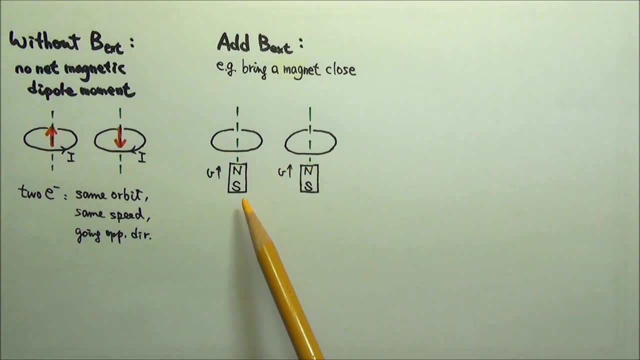 Now let's add an external magnetic field, For example by bringing a magnet close to the loop. Which direction-induced current will we have in these loops? The magnetic field is added, so the magnetic flux increases and the original magnetic field and the induced current's magnetic field should be in opposite directions. 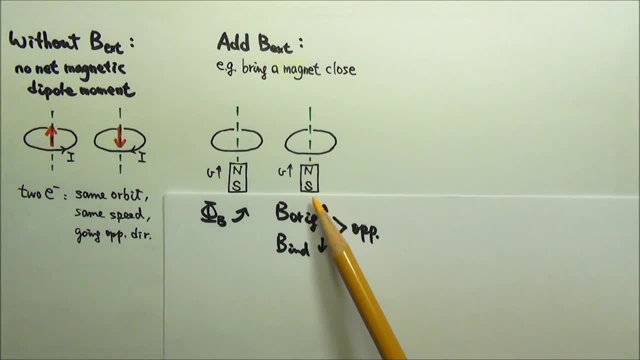 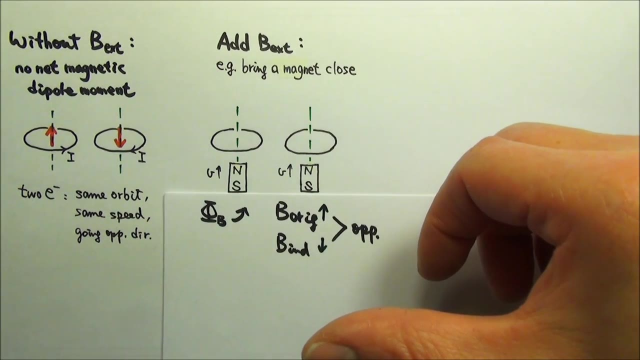 The original magnetic field produced by the magnet goes into the site out of the north, so it's upward. Therefore the induced current's magnetic field goes down. With the curved four fingers going down inside the loop, my thumb goes to the left. 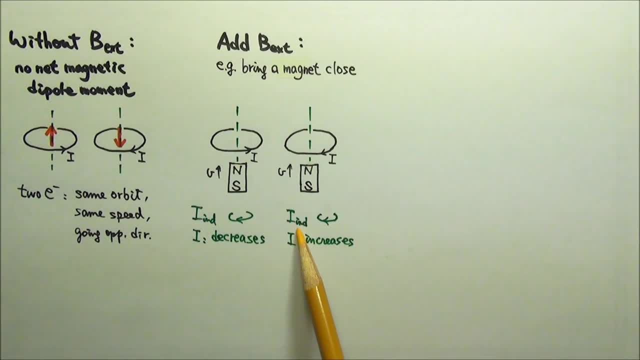 in the front. So the induced current is clockwise in both loops. Since the orbiting electrons already produce these currents, the induced current would cause the counterclockwise current to decrease and the clockwise current to increase. So induction causes this magnetic moment to. 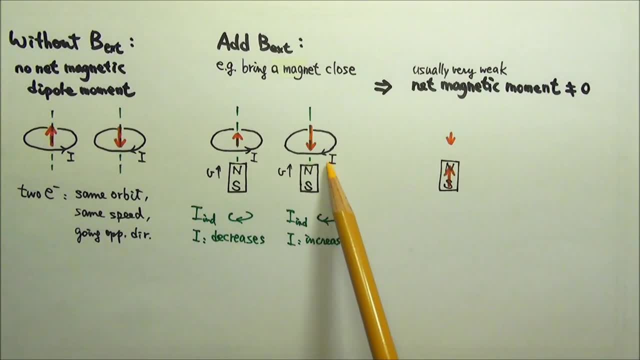 decrease slightly and that magnetic moment to increase slightly, resulting in a usually very weak net magnetic moment. that is the opposite in direction to the external magnetic field. Since this net downward magnetic moment is like a magnet, with north at the lower end, the material gets repelled by the magnet. 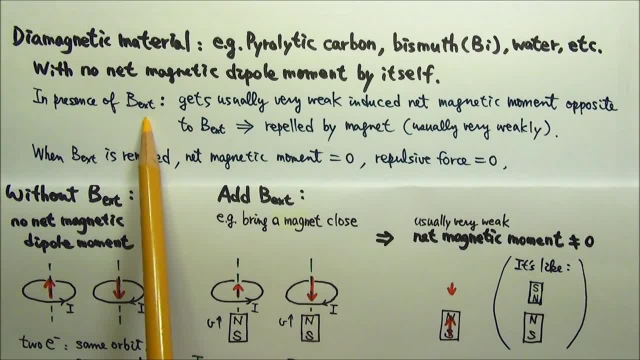 That's why, in the presence of external magnetic field a diamagnetic material gets a usually very weak induced net magnetic moment opposite in direction to the external magnetic field. So a jammed magnetic moment is repelled by a magnet, usually very weakly And when the